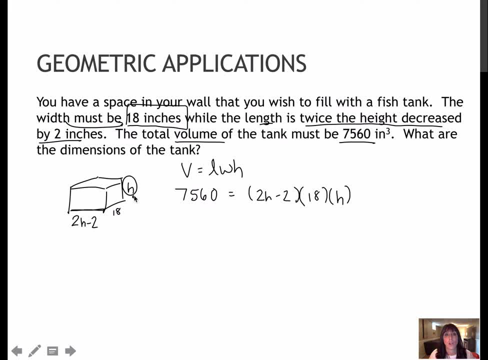 second unknown in relationship to the unknown that I had to begin with. So now it's just a matter of doing the math. I'm going to multiply all of this out, so I'm going to take 18 times h and then distribute it to both terms. So 18h times 2h is 36h squared, and then 18h times minus 2. 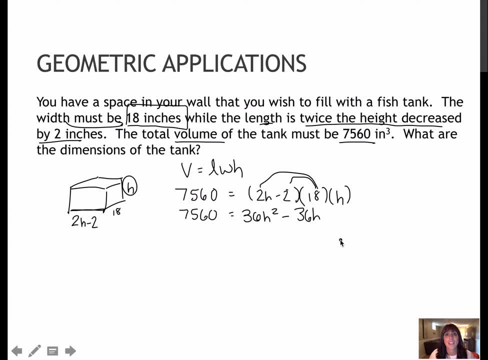 is minus 36h. I, of course, want everything on the same side of the equal sign, so I'm going to subtract the equal sign. I'm going to subtract the equal sign and then I'm going to subtract the 7,560 over to the other side. And I don't like- oops, it's a minus. I don't like the fact that 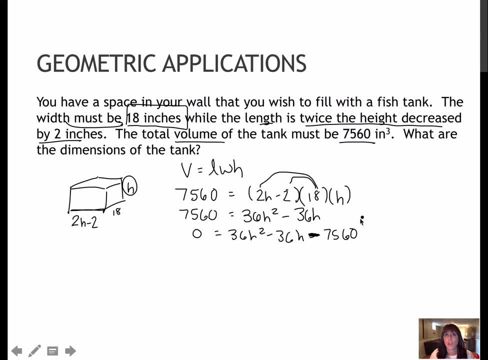 I've got these very, very large numbers to deal with, because that will make it hard to factor and even hard to use the quadratic formula. So I'm going to factor a 36 out of everything and that gives me h squared minus h, and 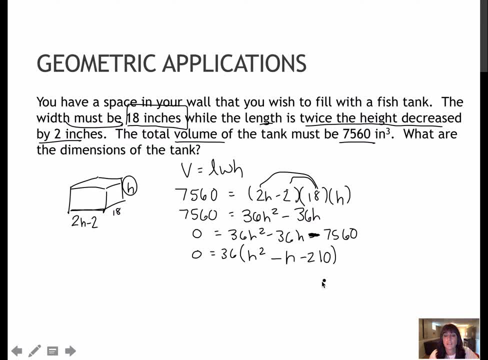 minus 210, equal to zero. That makes it much easier. Now I'm looking for numbers that multiply to 210, that have a difference of 1, and that turns out to be 14 and 15. And so it's h minus 15, h plus. 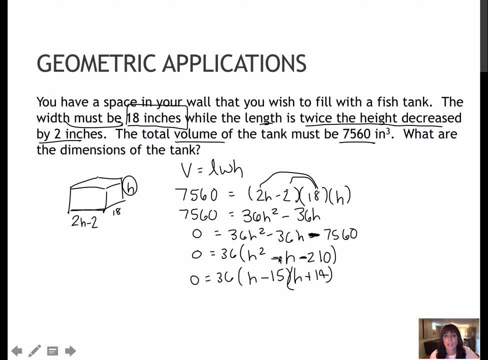 14,, because they had different signs and the larger number was negative, which means setting each of these equal to zero. I would find that h is positive 15, and I would find that h is positive 15, and h is negative 14.. Now, of course, this is a story problem, so it does not make sense. 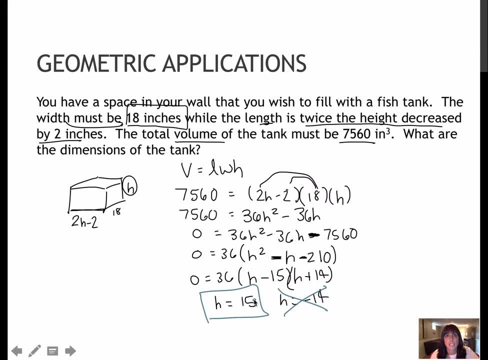 to have a negative answer. So I know that h is 15.. However, this asks for the dimensions of the tank, A little extra line in there. Dimensions of the tank would be h, which is 15 inches by 18 inches, by 2h minus 2.. So if h is 15, that's 2 times 15, which is 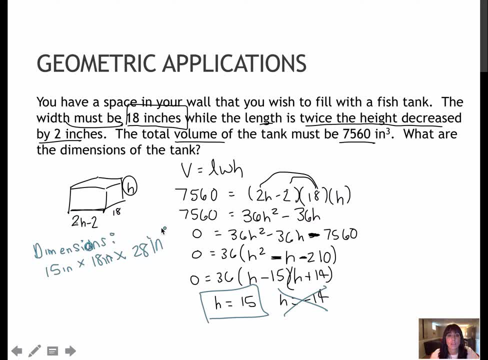 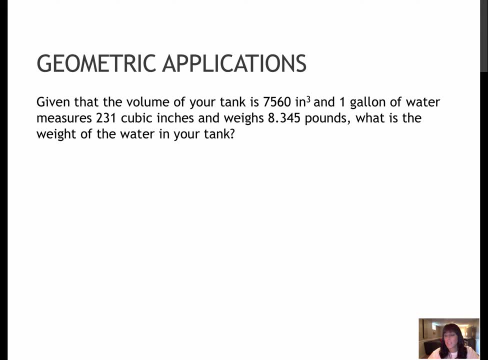 30 minus 2, or 28 inches. So those are the dimensions of the tank Used in that same example. we know that the volume of the tank is 7,560 cubic inches, and one gallon of water, which is the same as 231 cubic inches, weighs 8.345 pounds. We're. 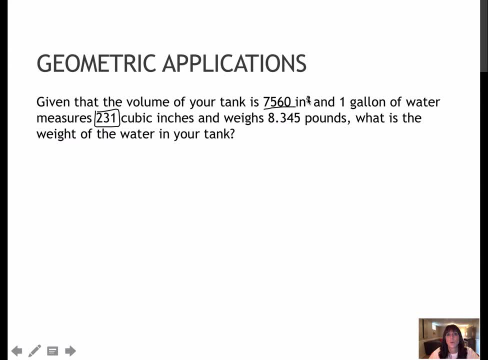 trying to find what's the weight of the water in our tank. So it makes sense that I'm going to turn this value, my volume, into gallons, so that I can multiply that by how much a gallon weighs. So I'm going to take 7,560 cubic inches. 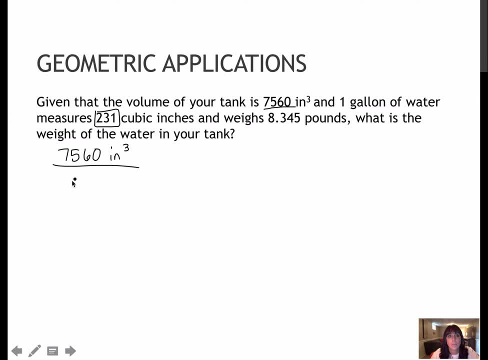 divided by well, I'll just say over one and then I'll say times 231 cubic inches to one gallon. Now notice: what will happen is that the inches cubed will cancel and my answer will be in gallons. Dividing that or multiplying, and dividing gives me an answer. 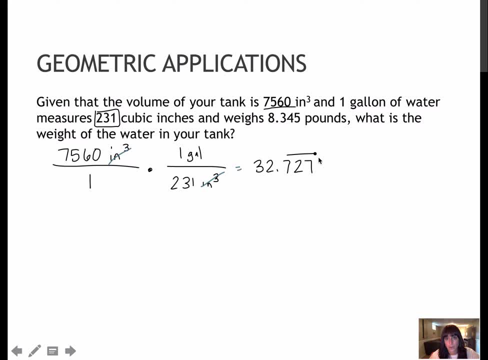 of 32.727, etc. repeating. Typically, I will leave that value in my calculator. Now I have gallons and I know that each of those weighs 8.345 pounds. so then I'm going to multiply that times 8.345, and that should give me pounds. I end up with about 273.1 pounds. so that would be. 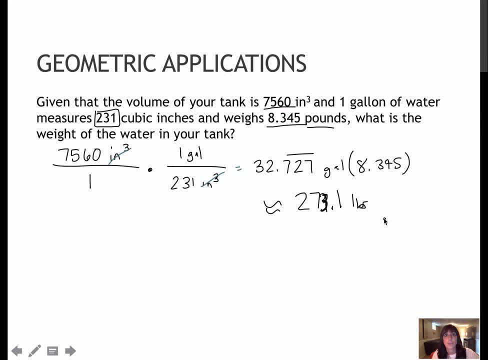 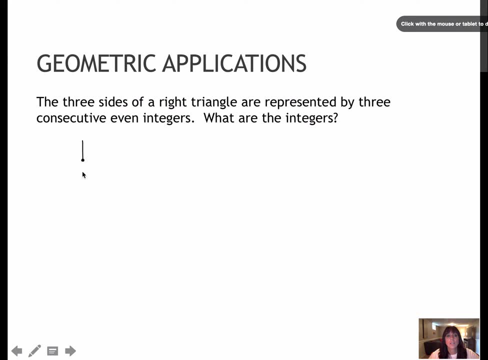 the answer to my question is way too heavy for me to carry by myself. We have three sides of a right triangle, so never a bad idea to make yourself a little picture: Three sides of a right triangle. Three sides of a right triangle. right triangle are represented by three consecutive, even integers, So consecutive. 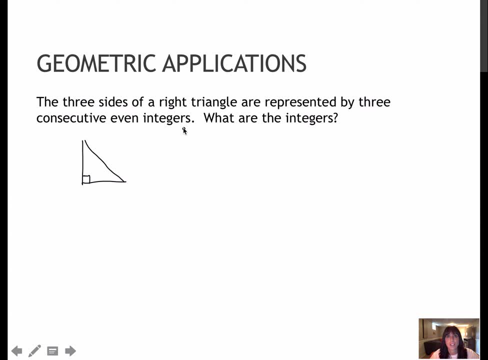 meaning in a row integers meaning there's no fractions, decimals, etc. So if I say that x is the first integer and they're even integers, even integers are two units apart. Two to four would be two units apart. Four to six is two units. 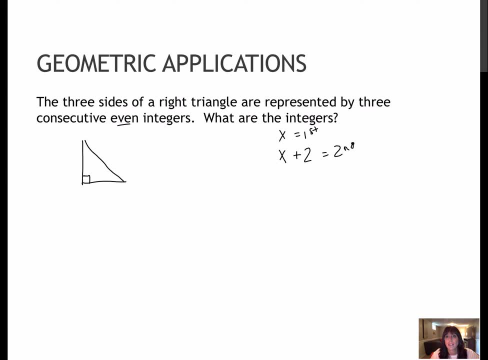 apart. So I'm going to say that x plus two is my second, and two more than x plus two, which is x plus four, is my third. Now I know in a right triangle the longest side is the hypotenuse. So this is x plus four, and then it doesn't. 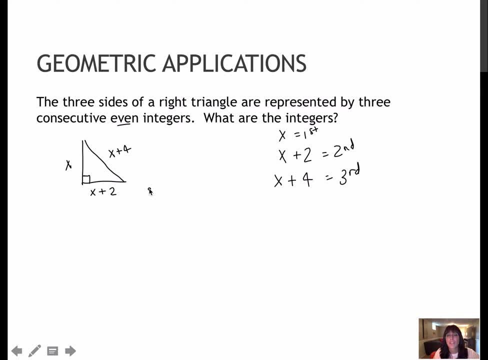 matter which one is x or x plus two. Another thing I know about right triangles is that they use the Pythagorean theorem, which is: leg squared plus leg squared equals hypotenuse squared. So x squared plus x plus two squared, those are the two legs equals x plus four squared, and that's the. 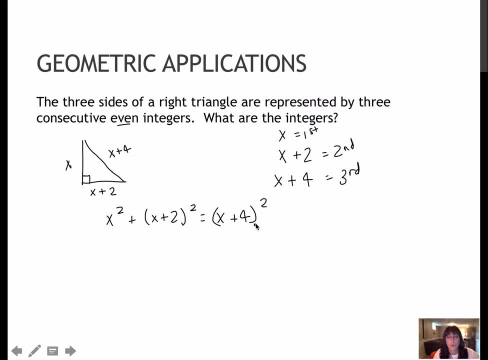 Pythagorean theorem. So now I'm just going to, you know, foil everything out. Remember, this is x squared, This is not x squared plus four. What we do is we take x plus two times x plus two and foil it out. So that's what that means is take that twice and then. 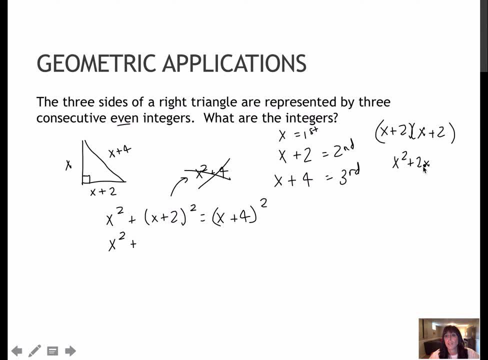 foil it out. So that would be x squared plus two, x plus two, x Plus four, which would of course be x squared plus four, x plus four. Doing the same thing over here, I would get x squared plus 8x plus 16. And I need to. 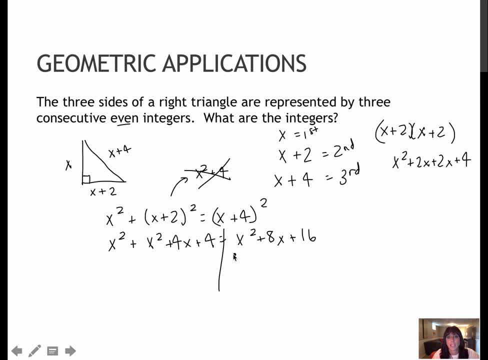 get everything to one side. So I'm going to get rid of this x squared, I'm going to get rid of the 8x, I'm going to get rid of the 16.. And on the right side, I just have zero, which is what I wanted. On the left side, I just have zero. And on the 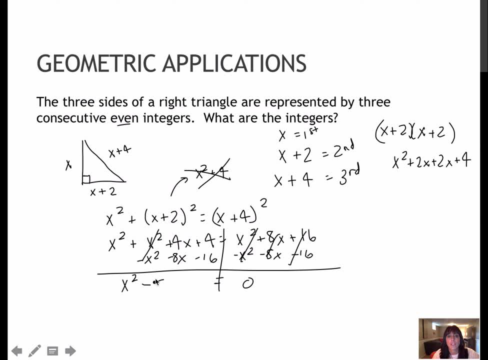 right side I just have zero, And on the left side I just have zero, And on the right side I have x squared, I have minus 4x and I have minus 12.. This does happen to factor into x minus 6, x plus 2, which would give me my two solutions of x equals 6 and x equals negative. 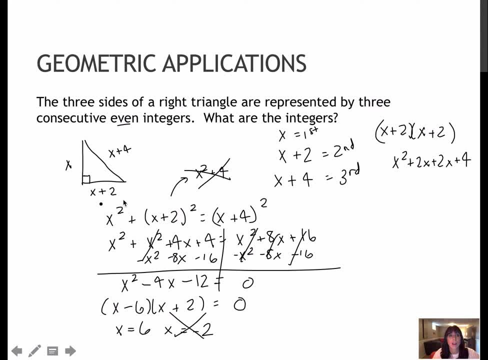 two. Again, the negative two would not make sense because we're talking about lengths and I couldn't have a length of negative two. So the integers are six and then x plus two, x plus two would be eight and x plus four would be ten. So the lengths of the triangle. 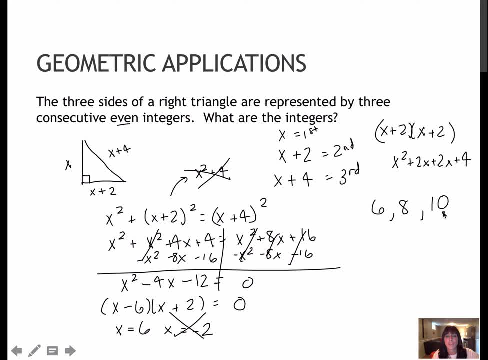 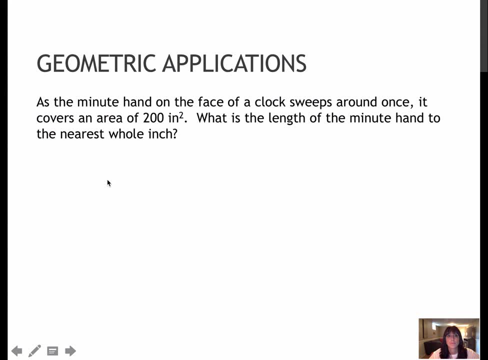 are six, eight and ten. They don't specify if they're inches or feet etc. But those are the integers used for the lengths of the triangle, This one's having to do with the circle. So we have a clock face and the minute hand. 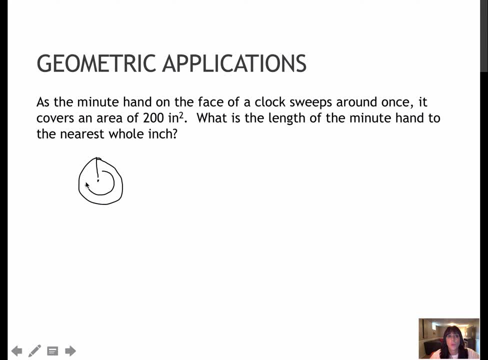 which, of course, is the long one. When it goes all the way around, it covers an area of 200 square inches, which is them telling us that the area of the circle is 200 square inches. They're asking what is the length of the minute hand. So the minute hand is the whole length. 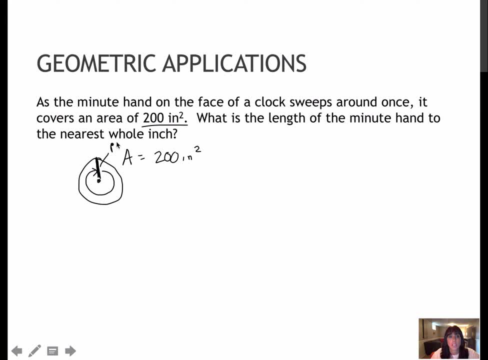 of the clock from the center, which of course is a radius. So essentially they're saying: here's the area, find the radius. We know that the area of a circle is pi r squared, so that's the formula we will use. They give us that the area is 200.. Pi, we're just going. 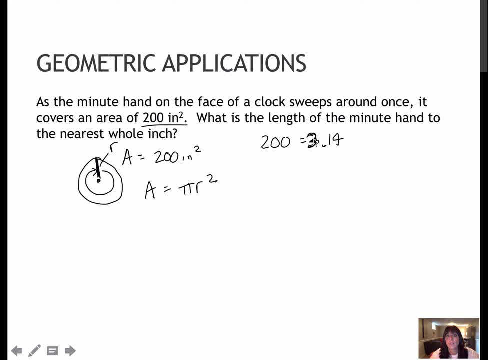 to use 3.14 and radius squared- we don't know. I'll divide each side by 3.14, which of course will give me r squared all by itself. over here On this side, I get 63.69, etc. I leave. 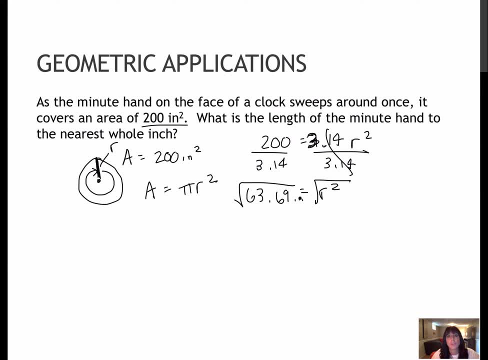 that entire decimal in my calculator and then I will take the square root of it And that gives me, rounded to the nearest whole inch, about 8 inches. So about 8 inches would be the radius, a little bit less than 8.. 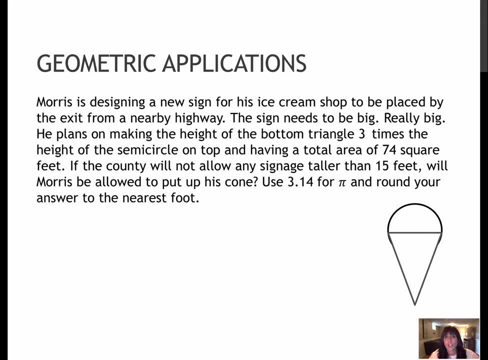 Here's an ice cream shop. He wants a very large ice cream for his sign, but the county says: make sure that it's not taller than 15 feet. So our job is to determine if he can have this ice cream cone, based on all of his signs. 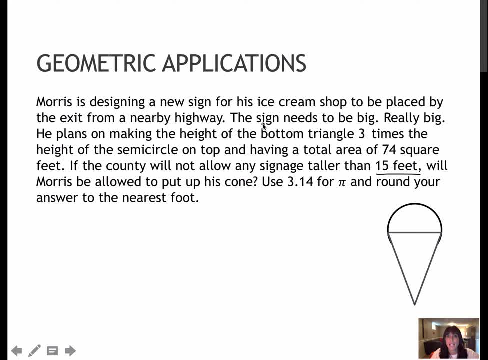 So the sign needs to be big. the height of the bottom triangle is 3 times the height of the semicircle on top. So if this distance, which is of course the radius, would be x, then this distance would be 3x, because it would be 3 times the height of the smaller. 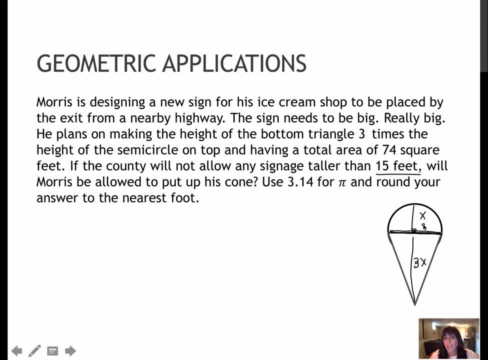 And, of course, this distance all the way across would be 2x, because it would be 2 times the radius. So now we have everything we need to figure out the area, or to figure out the x's based on the total area of 74 square feet. So first let's just look at the area of each. 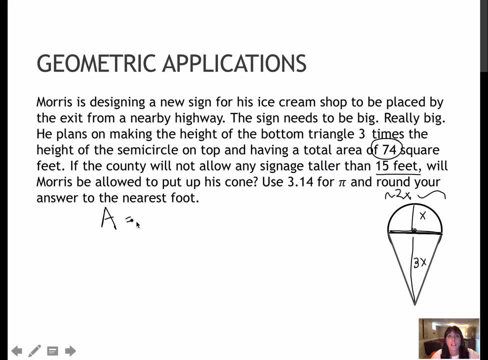 of these parts of the figure If I were to find the area of the figure. this is a semicircle, so half of a circle. A circle is pi r squared. I'm going to take half of that. A triangle is 1 half. 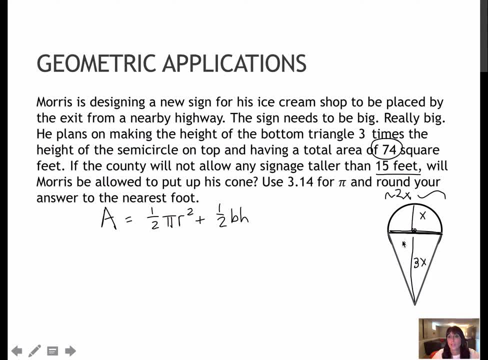 times base times height. So that's how I'm going to find the area, And now I'm going to plug in the values that I know. Area is 74, 1 half times 3.14 times r squared, which in our case is 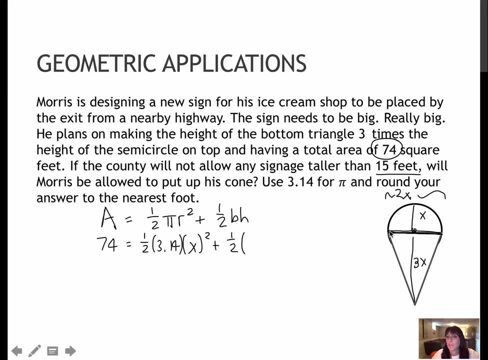 x squared, And then 1 half times the base, which we said was 2x, times the height, which we said is 3x. So those are all of the values and of course, our only unknown is x, The last. one is going to be 74, so we have 3 x squared. That's what we're going to do now. So I'm going to go ahead and swap out the value into the value of the cross, The cost that I'm going. to be asking to do is 1.17 x squared plus 3 x squared. I'm going to leave that at 1.17.. And now we have the threshold value, 4.55 x squared, which is 4.57 x squared. so that's. 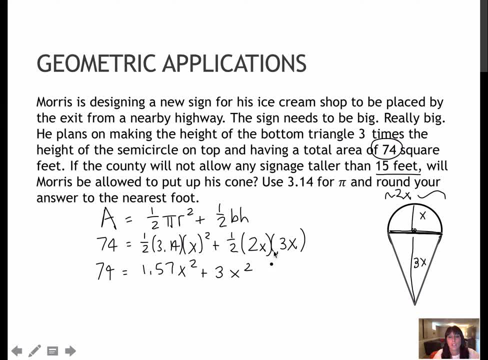 what I'm going to do. So that's 1.17 x squared plus 3 x squared. Notice, there's no x to the first value. So in this case I will not move the 74 over. I'm going to leave the 74 on. 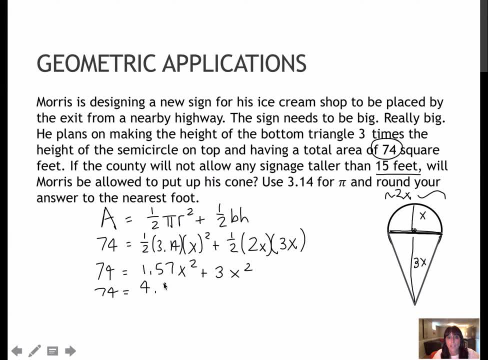 the left. I'll combine like terms over here, so 4.57 x squared. I'll divide both sides by 4.57.. That leaves me with x squared equals 1.57 x squared. This is the minimum value we're. 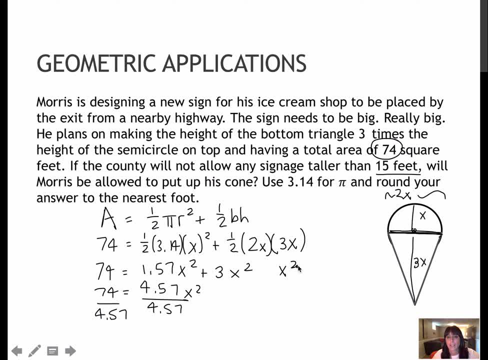 that leaves me with x squared equals about 16.19. again, I'll leave that decimal in my calculator. take the square root of each side and get that x is about four point zero two. I'm going to round that answer to the nearest foot, so I'm going to say it's about four feet. but the question says: can he put up his? 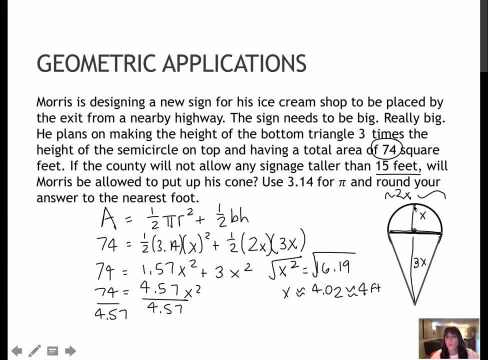 cone, if X is 4. so if X is 4, then that means this distance is 4 and this distance is 12, leaving us with a total height of 4 plus 12 or 16 feet. they won't let us have anything taller than 15 feet. so no, sorry Morris, you can't. 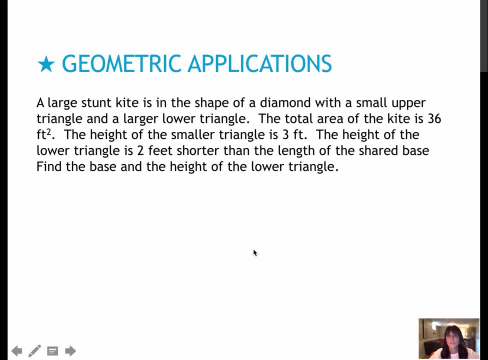 have your sign. this last question is one for you to do on your own. this is one very similar to our last question, so press pause, try this question and then press play to see how you did. here we have basically a kite that's in a diamond shape. it tells us that the 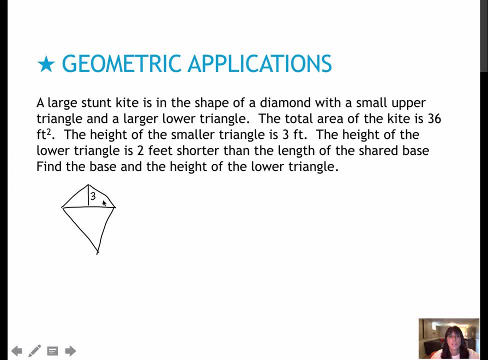 height of this smaller triangle is 3 feet. it tells us that the height of the lower triangle is 2 feet shorter than the length of the shared base. so let's call this shared base X, that's all the way across. is X the height of this? 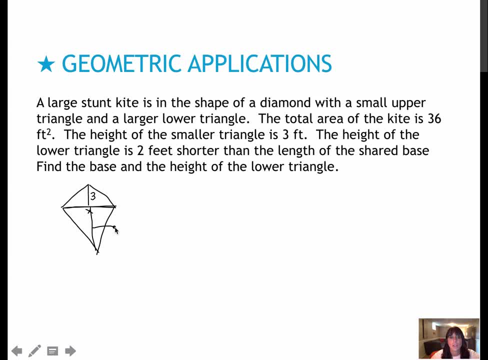 triangle is two feet shorter than that, so this is going to be x minus two. To find the area of this figure, I'd have to find the area of two different triangles. So the area which they've told us is 36 square feet is equal to one half base times height of the smaller triangle, so the base is x. 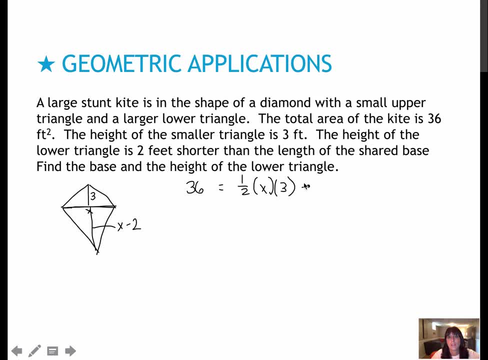 the height is three. The area of the larger triangle is one half base times height of the larger. so the base of the larger is x and the height of the larger is x minus two. From here we're just going to do a lot of multiplication. I see that I've got a lot of 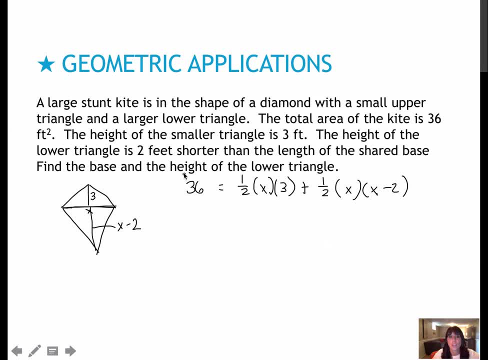 one halves here. I don't love dealing with fractions, so a little trick on clearing fractions is to take each term by two. So by doing that on the left side that just gives me 72.. On the right side that leaves me with. 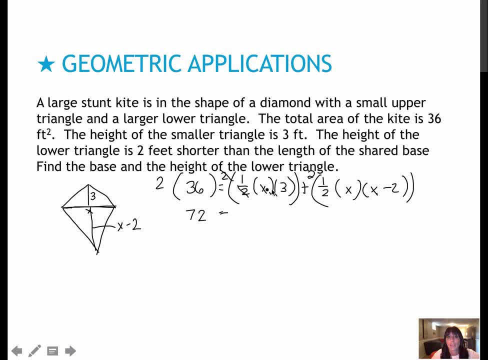 the one half and the two going away, giving me x times three or three x, and then, on this one, of course, the one half and the two going away, giving me x squared minus two x. So much, much easier than dealing with the one halves all the way through the. 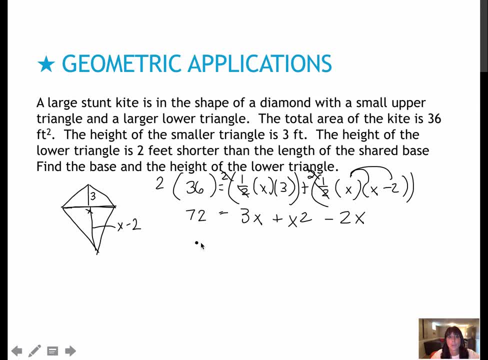 question. This one does have an x squared and an x term, so everything's going to go to one side, meaning I'm going to subtract 72 from each side and do some rearranging. I have x squared, I have plus x.